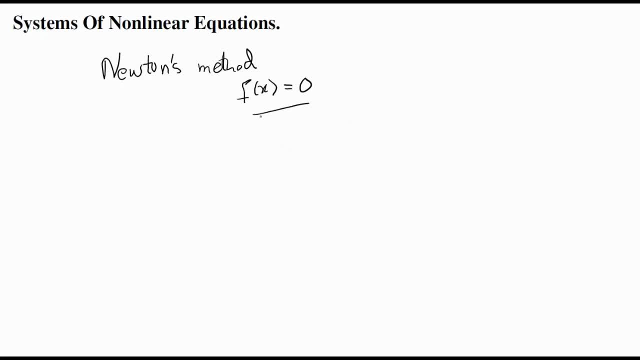 equation and it could be anything. It could be sine x, cos x, any combination of functions just is equal to zero, And the method of solution we looked at was that xn plus one equals xn. it's an iterative method and it's just a function f at xn divided. 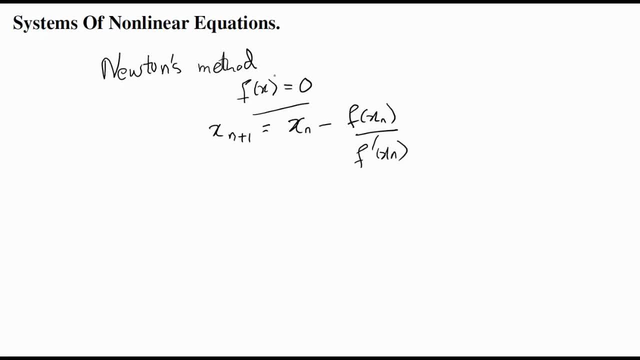 by f, dash, xn, And basically we're looking for the x's which satisfy this basic equation. So that was Newton's method. Now, then, after that, we've looked at, of course, systems of equations, And a system of equations, remember, means when you're solving simultaneous. 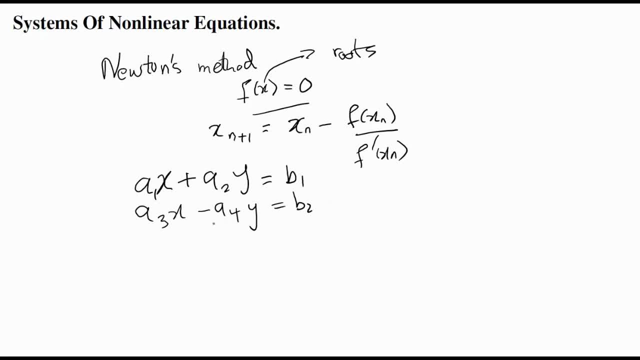 equations. So we've been looking at, for instance, simultaneous equations, So two or more basically, equations form a system of equations. Now, in this particular topic here, we're looking at systems of non-linear equations. So basically what we are going. 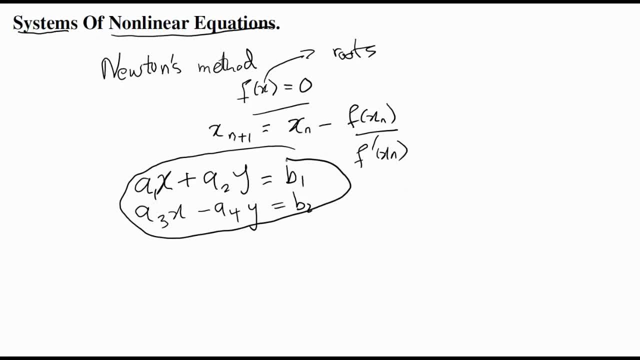 to be doing is, instead of you know these types of equations, we're looking at a combination of a bunch of these types of equations forming a system. So that means that we're not going to be looking at just one function, but we're going to say: well, f1 x equals zero. So 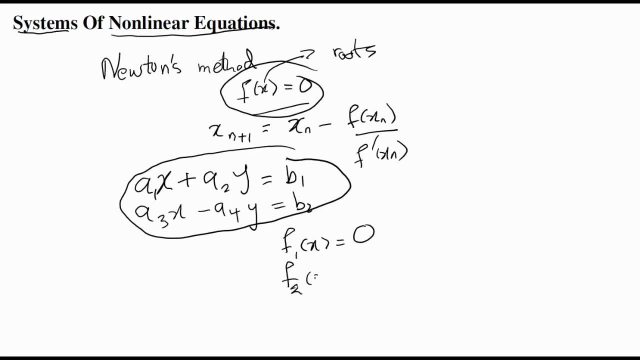 f1 x equals zero, f2 x equals zero, And so on and so on, up to some function: fn equal to zero. So we're going to look at a bunch of non-linear equations. So what do these equations actually look like? Example would be, for instance: now: instead of x plus y, 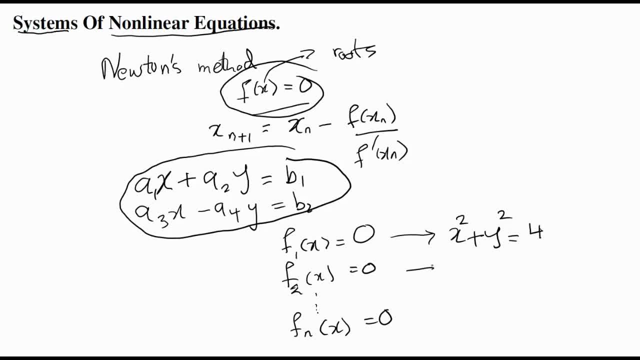 we might be looking at: x squared plus y squared equals 4.. And another equation could be: with it: x minus y equals 7.. Now we are going to limit our. we are going to limit ourselves to just a system of non-linear algebraic equations. Okay, So we're going to limit ourselves to non-linear algebraic. 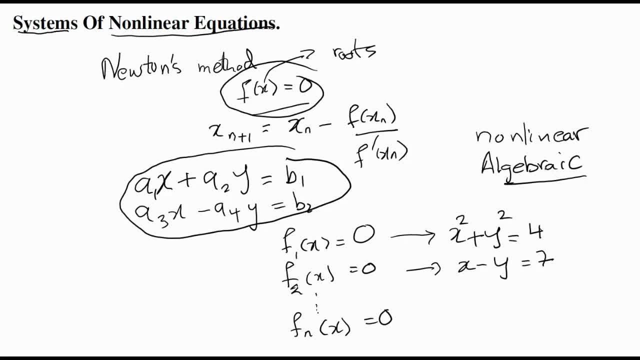 equations, Because if we say non-linear generally that could mean anything. So for the to limit ourselves, we're going to just be looking at a method that actually looks at, and we're going to consider looking at non-linear algebraic equations. 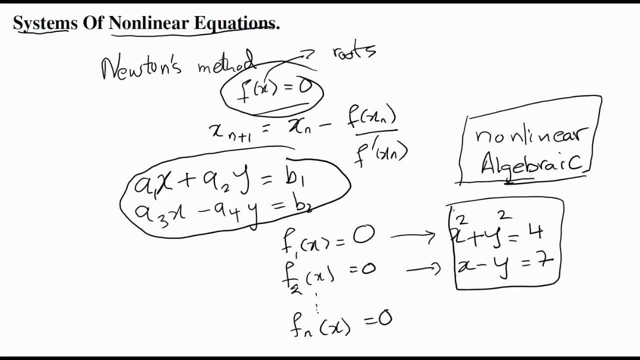 So this would be a good example of that. okay, is you have some x squared plus y squared, or x cubed plus y cubed, and so on and so forth, And they've got it right inside Now, of course, it's very these equations. another thing we need to keep in mind is this is how we 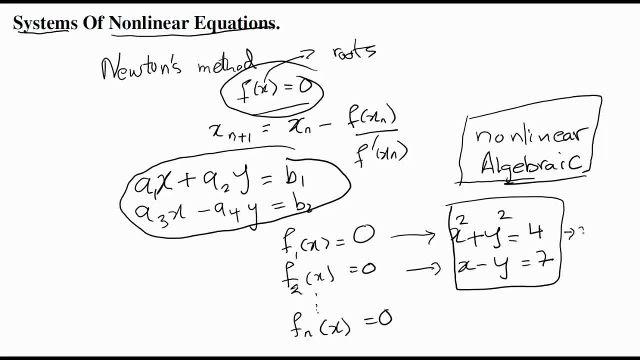 were looking at the equations. We're now going to try to do the following, which is we're going to rewrite this as: x squared plus y, squared minus 4, equals zero. Okay, So that, and this one, for instance, would be: x squared plus y, squared minus 4, equals zero. Okay. 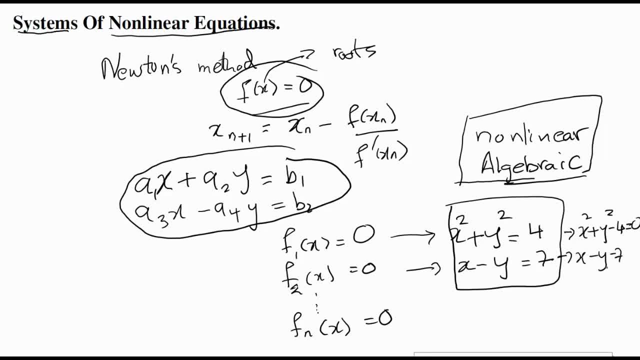 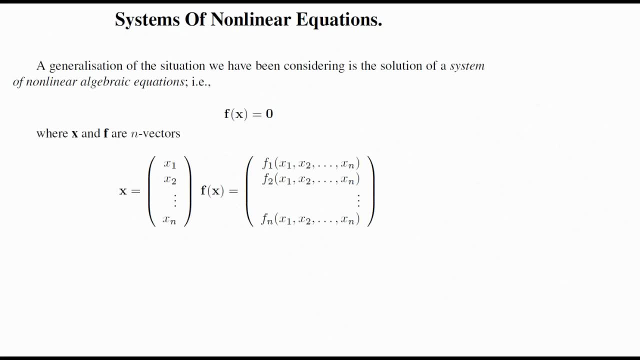 So the next would be similar: x minus y minus 7, okay, equals zero. So if you look at this, that's the kind of that's what we mean by systems of non-linear equations, Okay, So here's just things a little bit cleaned up now. So basically, you can see, there's your. 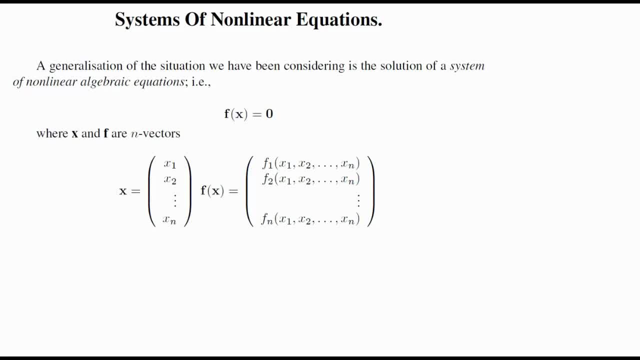 so f is the vector. now, Okay, Here f is the vector And basically, but F, here, this, this is the vector, This is the one, this is the dynamic input autonomous parts of the equation. The other two requested: This is the apartment lot and four is the momentary. 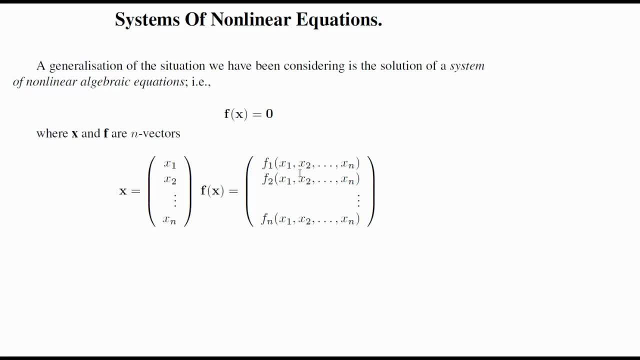 momentary increase effectively due to dispersed pressure. the document of infinity or invariant. this is what i was talking about, the f1, f2, which are functions of uh, different variables, x1, x2 up to xn, uh, the x vector here shows you the number of variables you have, like in the example i had. 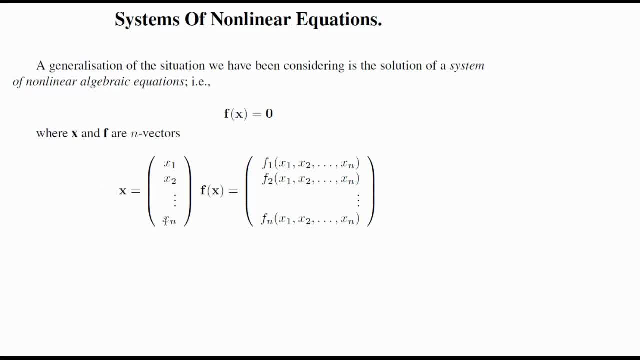 an x and a y, so that's just a two variable, two function uh system. so here you have n functions and you've got, of course, n variables uh that these functions seem to be depending on. so as we put uh things together, basically uh to look at some notation, now it's going to be vector functions. so 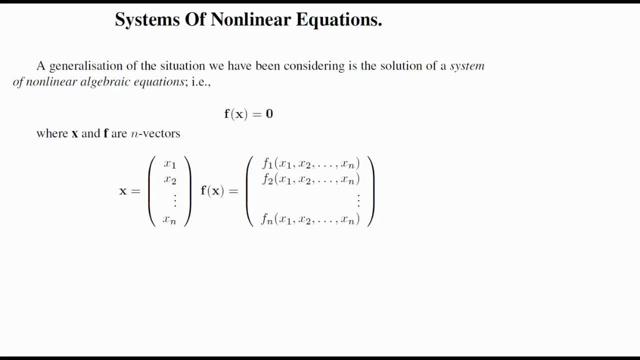 these vector functions equal to zero vector. so the zero on this side that you see, this is the zero vector, essentially, and f here is basically got this structure on it. so that's what, uh, so that's what we're formally talking about. so how does one solve this? well, let me just uh on the side here. 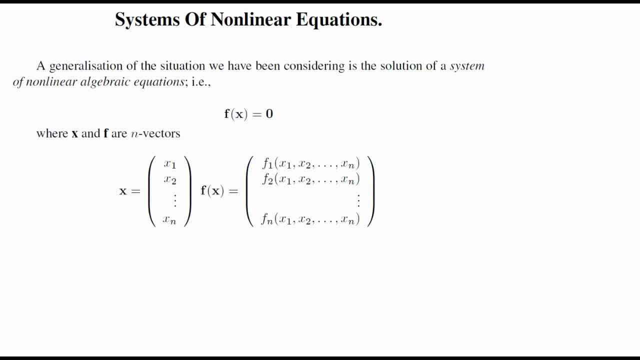 show you, uh, reminding you again- which i did just before- that we looked at, of course, uh, newton's method and newton's method, uh, again. now, that was newton's method. so in this case, if we were to implement newton's method, so the vector version of this could possibly be, for instance, so i'll have the vector. 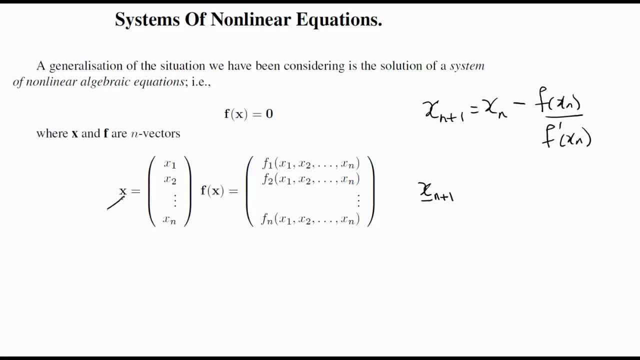 x n plus 1, where vector x is this vector here. now that's going to be equal to the vector x n. so at step x n plus 1 equals step x n, but it's a vector. now i'm looking at that's not a problem. so far, so good, and we look at the vector function at the step vector x n. 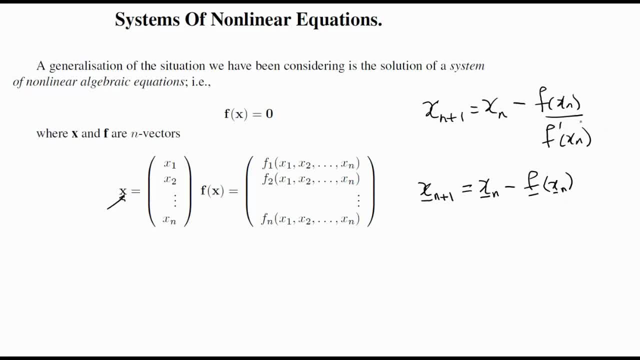 now that all looks fine. the problem is: is this, uh, this division, uh, by f dash now, what is f dash now? remember we're talking about vectors, first of all vectors and matrices. the concept of division is not the same as uh division here, with the something over something. we can't do that. 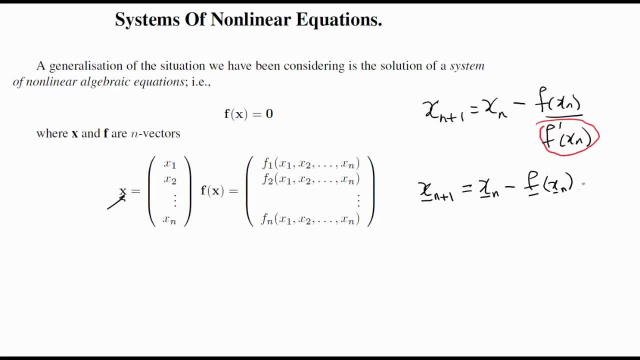 so what is the equivalent of uh? division is actually the inverse. so we're looking at, basically we want to figure out, first of all, what is a vector containing the derivatives of the function f, something? and it's. it's exactly there where we introduce now the concept of something called the jacobian. now, you might have seen this before when you studied. 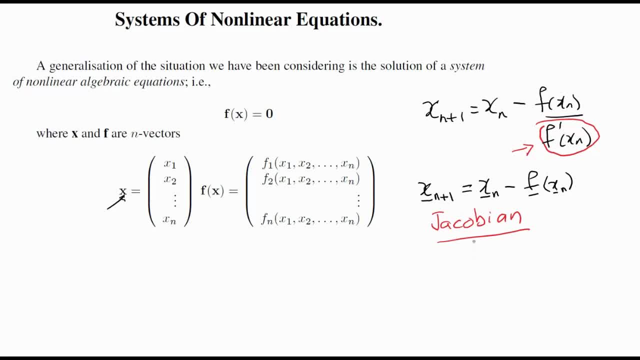 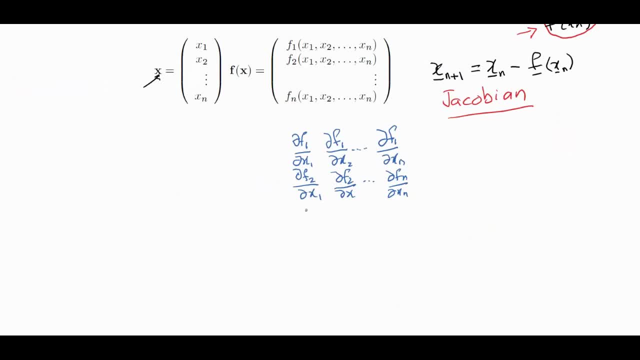 vector functions perhaps, but uh, the concept is very straightforward. uh, let me just show you what we are really talking about. so this would this would go on down all the way up to the nth function, okay, x1, and then fx and uh and f3, fn divided by x. 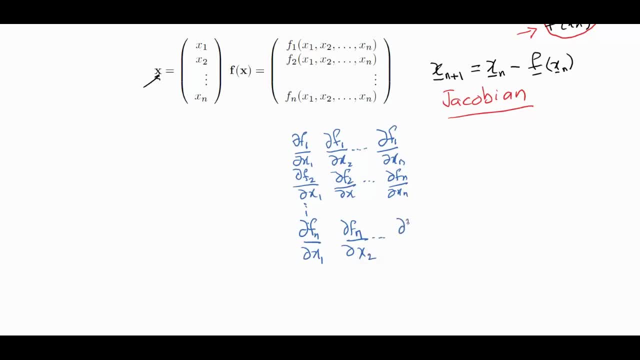 x2, x2 and then all the way to fn, x, uh, sorry, xn, so that this, uh, rather this matrix, this is called the jacobian, this is called the jacobian. so the jacobian is something that basically represents the equivalent of the derivative that we had in newton's method. so let's clean this up a little. 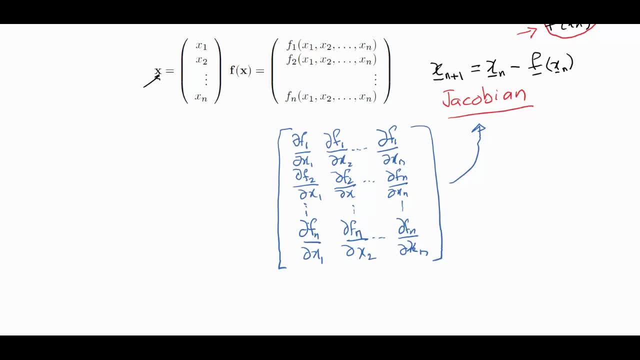 bit and uh, look at what happens next. okay, so here's the jacobian matrix, just cleaned up a little bit, um, and now what remains is how do we incorporate that basically into, uh, for instance here: as you looked at, this was: this is newton's method, so we have this. 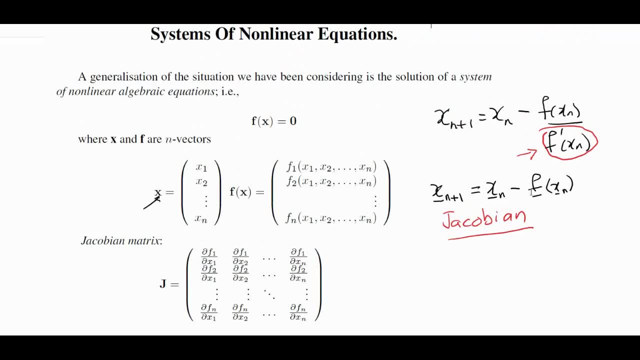 f, dash x out. so obviously, one thing that occurs to quickly to mind is that we're going to take the inverse of this matrix. okay, if that's the jacobian, that's the derivative, then if i take the um, the inverse of this matrix, and multiply it into this, so what i'm saying is something like: 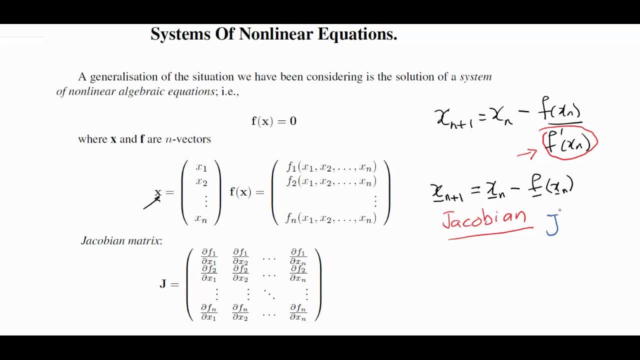 the j inverse. so if i were to multiply this uh by j inverse at, of course, xn, uh, which was, which is a matrix, of course, and put that here, okay, because i can't put it here. so if i put that here, no, so if i put that here somehow, then i can't put it here. so if i put that here, no, so if i put that here somehow, then 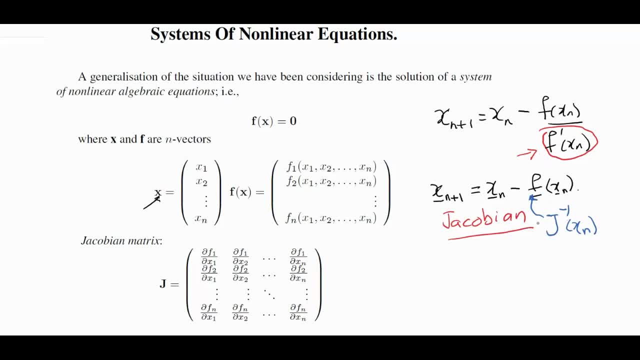 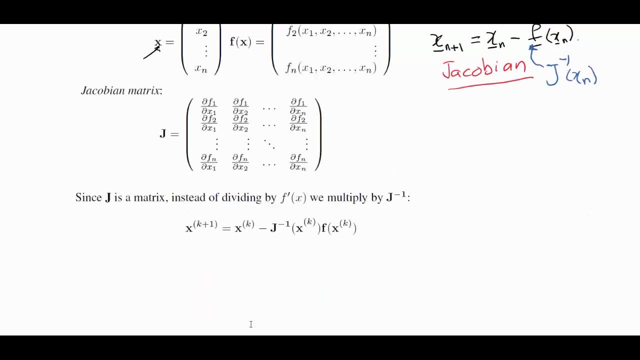 i should be able to in fact have an, have a, have a newton's method, uh, a systems version of systems of equations. let's just look at this in a little bit more detail now. so, basically, this method works reasonably well. the only thing we need to now know is: uh, we need, and, of course, 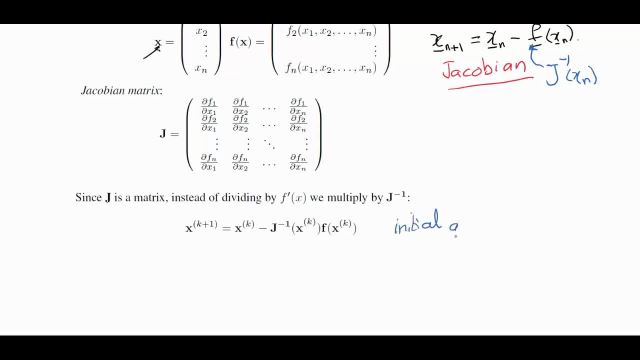 an initial guess, and the initial guess- uh, of course, as usual, is a vector, and this time it's going to be in the form of a vector, so we're going to leave it there. and it's now showing us this. of course, the idea of measured vibration is that, if we look at alsoano, which is a couple equations, uh, in this, 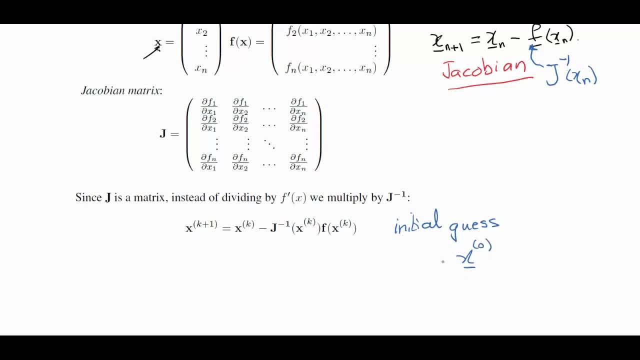 vector one, of course there's a different one, or, of course, and somewhere. so that gives us the idea of, of course, the initial guess, and then we'll take a look at the interval between the parts. so in this case, for instance, we call- we will refer to that as X, the zero step. now one thing: I 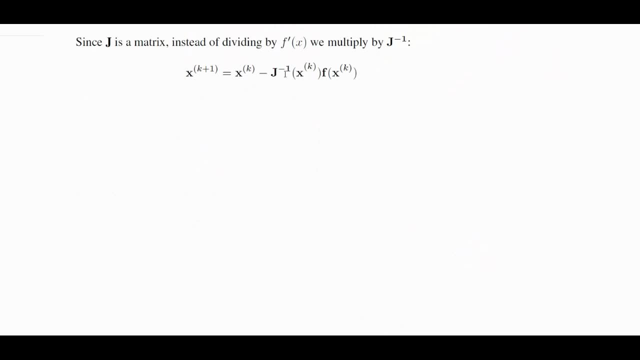 would point out is, if you remember now, although we have this inverse and it all looks very good, but remember, what we've learned so far from solving linear systems is that that is not a great idea. we should not have the inverse, because it's extremely difficult and not difficult, but it's very expensive to 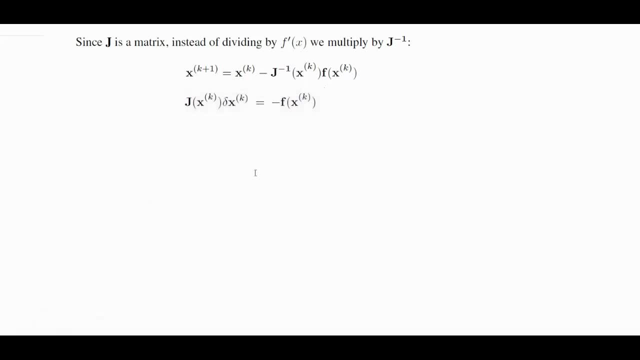 calculate. so instead of this, what we can do is just rearrange the equation, and we actually so. if we rearrange the equation, we end up with this, basically equation where this Delta X of K is just the difference between X K plus 1 and X K in. 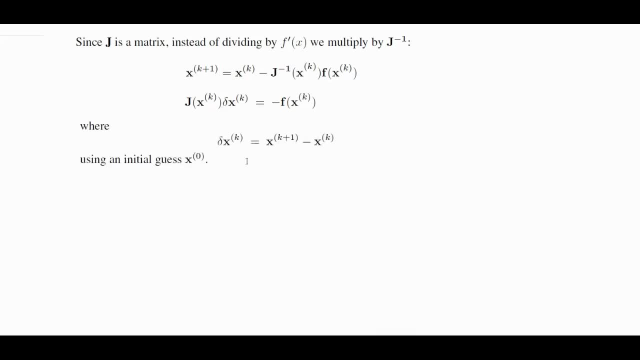 fact. so let me write that so where Delta X K is just X K plus 1 minus X K that you see here. so just take that to the other side, multiply across by the J inverse- a J inverse- which becomes J, a boat- multiply both sides of the equation and then you get the delta X of K, which is just the. 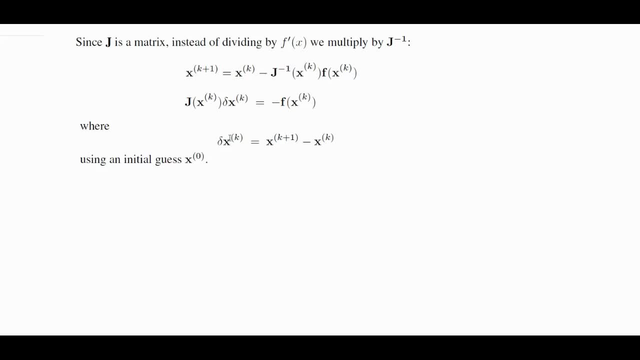 both sides, sorry by J, and you end up with this. so Delta X K- have just cleaned up things a little bit- is just X K plus 1 minus X K. so let's, we're now in a position to start looking at some examples. so here's an example. this is: 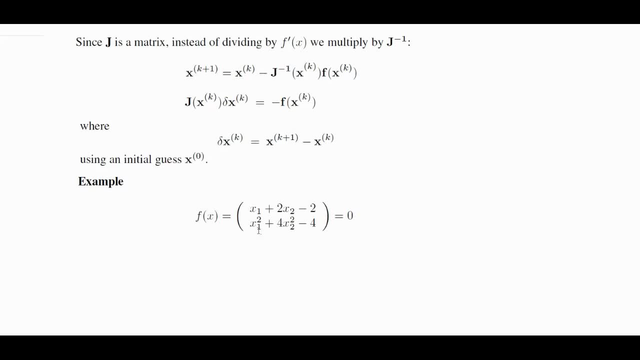 what typically what we would have. we've got a second equation. you see is non linear, clearly. so we want to solve the system of equations for the variables X 1 and X 2. so the first step, of course, would be to calculate the, the Jacobian. 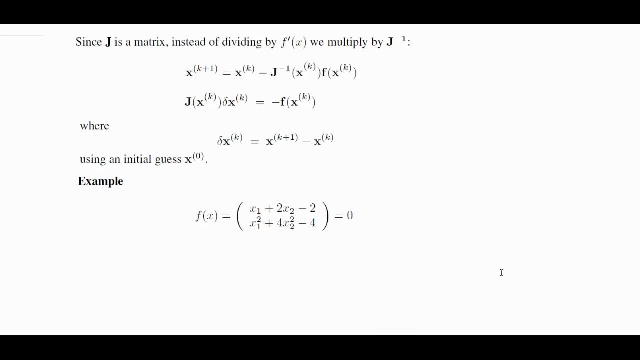 in this case. so that would mean that in the Jacobian' remember this, let me show you that- so the Jacobian of this matrix here, of course, it would mean that, and then the derivative of F1 with respect to X, two, which is 2, and then for f 2, the 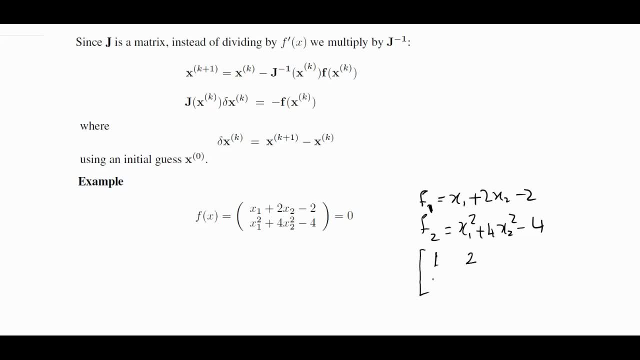 derivative of F 2, sorry, with respect to x1, which is gonna give me 2x1, and then the derivative of this whole thing with respect to X- 2. so that's going to be 0, that's going to be just 2x, 2 times 40 each. so you have to do 3x, 3x and 1x, 3x, 2x. we're going to do 3. 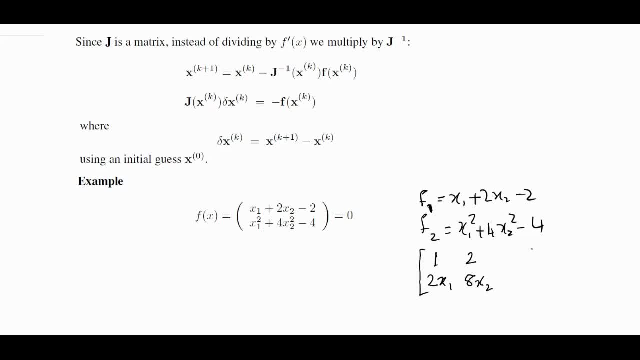 which is 8x2, and, of course, remember, 4 is a constant. so there's no uh, it's just going to be zero. so we end up with this: uh, jacobian. so they're uh, just uh, that's the jacobian. so in this case, for this particular matrix, as you see, 1, 2, 2x1 and 8x2. now we'll start the uh. now we'll. 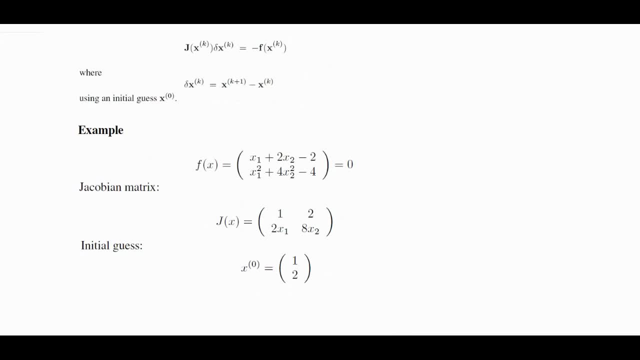 just set up our iterative process to start. so to start the iterative process, as you know, first thing we need is a, an initial guess. so we'll use this initial guess here. x of 0 equals 1- 2, so that means x1 is 1 and x2 is 2, so just let me indicate that here that's x1 and this here is x2. sorry, uh. 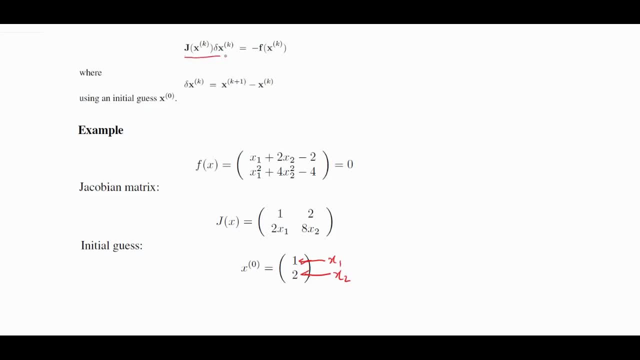 so, if i can just come back here and let's, let's look at this. this is the uh iterative process that we're working with. so so now we've got our initial guess. uh, let's look at uh, x, x2, x2 of j, the jacobian okay of x, of zero. so what's that going to be? 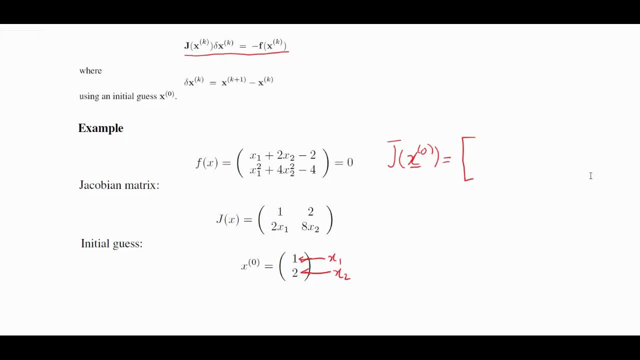 okay. so if we calculate the jacobian at the initial get x0, that means x1 is 1. first of all, these are just constants here, so that will just be 1 and that will be 2. they don't change. now. 2 times x1, x1 is 1, so that will be 2 times 1, which is 2. 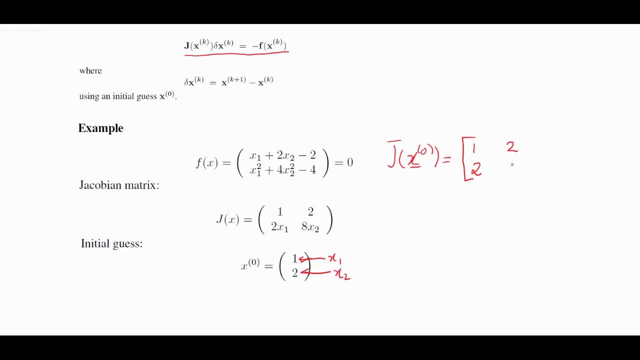 and then you'll have 8 times x2, and x2 is 2, so that will be 16, so that will give us basically the jacobian now next. so if we look here, now we've got the jacobian at x0. now the next thing we need. 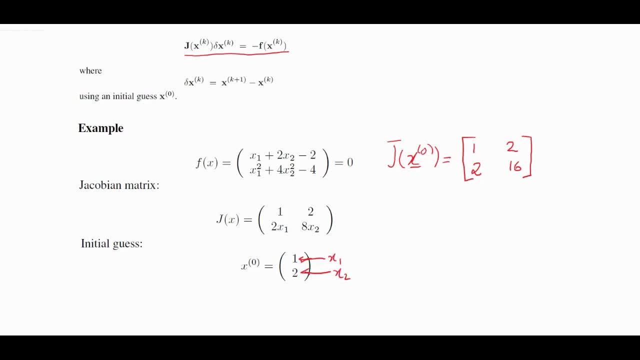 is this: uh, f at x0, so let's do that. so now, f, of course, is here, as you see, and what we're going to do is substitute for x1 1 and x2. uh is going to be 2 and we're going to substitute these values in here, so that means that that. 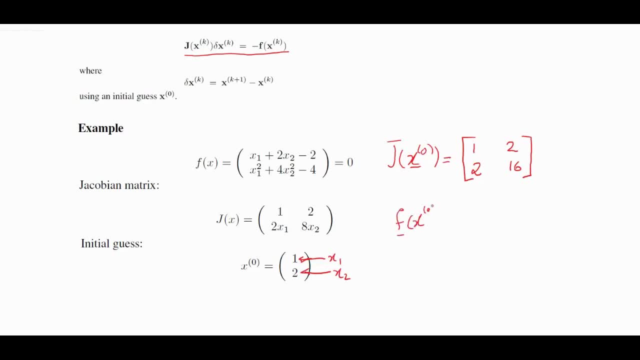 means that we'll have f at x0, okay, and that's going to be equal to. so first it's going to be x1, which is 1 plus uh 2x2, that's 4 minus 2, and then we'll have, of course, uh. x1 is 1 squared. so 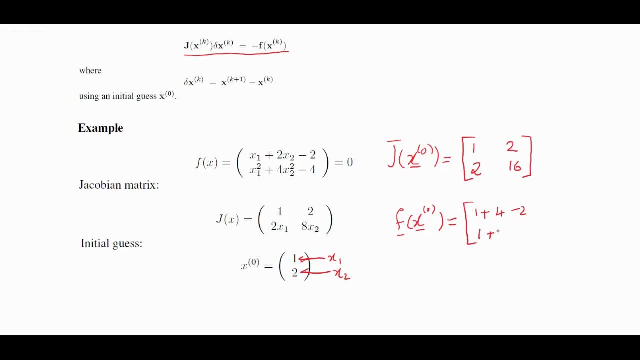 it's 1 plus 4 times x2 squared, which is 4 forces, and then we'll have a system called ax equals b. so remember this. compare this to the system ax equals b. now we've got b, our b is this here, okay? and our a. 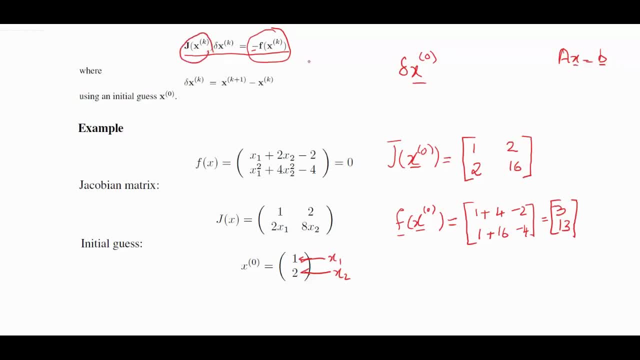 uh, okay, and our a is this over here. so that just leaves basically, uh, the, the, uh, sorry, this here, which will be our x, okay, so we're going to solve for this, so we're going to solve for this, and then we'll calculate. uh, our next iterate, which is x1. 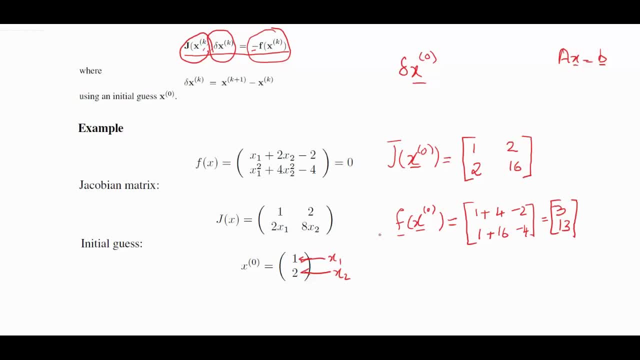 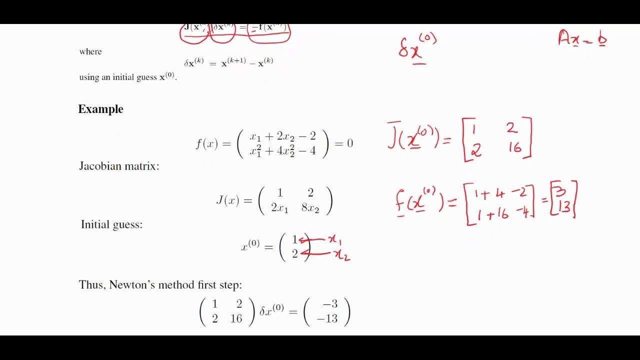 so I hope you understand that. so let's proceed. so here's everything just written for you all together. as you see, these are just the Jacobian and this F of at X, 0, and of course it's negative here, as you see, minus, so that they'll say minus 3 and minus 13. so that's basically now our equation. 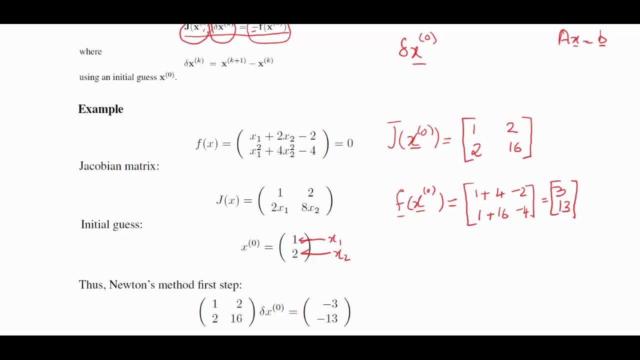 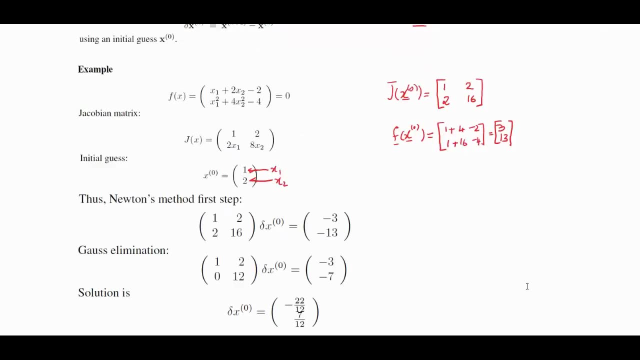 that we want to solve using Gaussian elimination. so we'll use Gaussian elimination to solve this for Delta X 0. next we apply Gaussian elimination. it gives us 1, 2, 0, 12, and then on the other side, minus 3, 7. so when we solve it we get this result now. so I just have rewritten it down here for you. 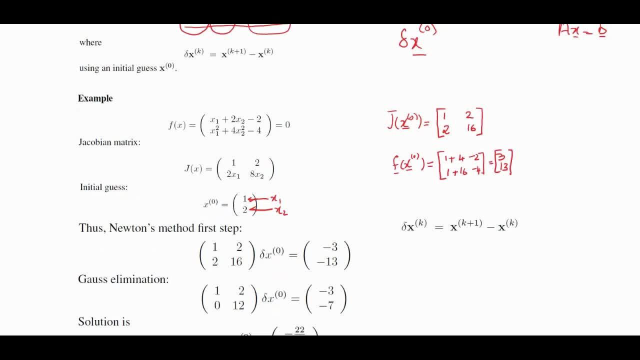 so you can see, this is what we're doing. so now, for in our case, of course, so Delta X 0, which we already have. so basically, what we're saying is that X 1, so X 1- okay, is going to be, of course, the Delta X zero that we have. so it'll be Delta X 0, okay, and plus X. 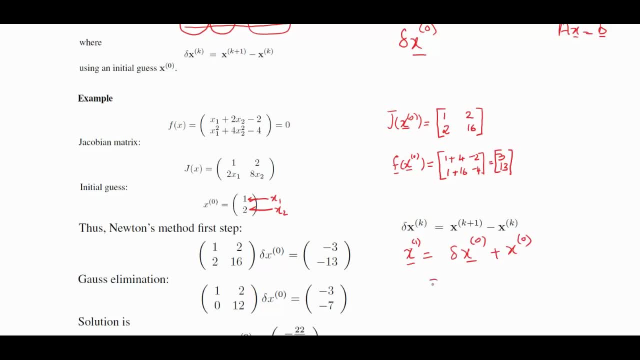 zero, okay. so now we already have Delta X: 0, it's minus 22 over 12 and 7 over 12, it's okay. and then plus we add that to 12, and so we get 12 over 12, and we get 12 over 12, and so we get 12 over 12, and so we get. 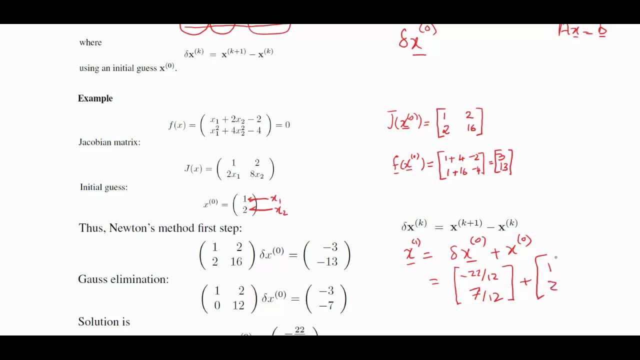 initial guess to that which we are using is one, two, and that gives us of course the final here. so that gives us minus 10 over 12 and 17 over 12.. so we've got our now the first iteration. so you see, it's sort of done in two steps. in the first step we calculate delta x0 using gaussian. 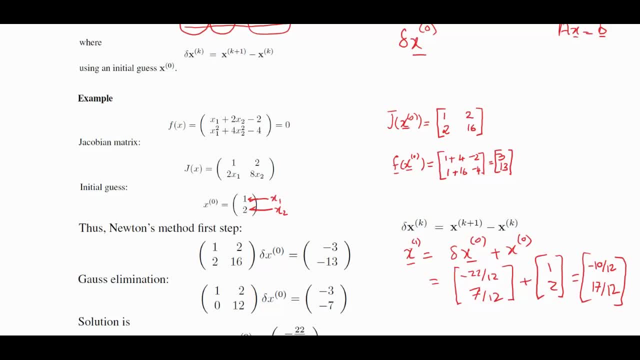 elimination, uh, as done here, and then we calculate x1. in fact, and that's the update, now that we have x1, we can proceed to calculate the next uh, the jacobian, at x1 and the, the function, at x1, just like we did uh here, as you saw here, uh at x0. so now we'll have x1. so this, this will be a new matrix. 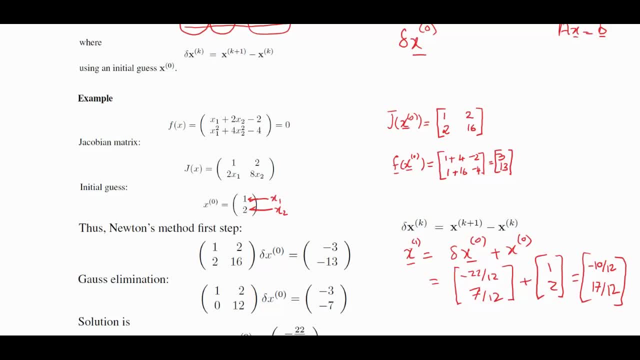 our function at x1 will get updated, and then, of course, we'll go through the same process, calculate delta x again, and and that's basically how this works. so let's just put everything together again. so here's just uh written down. so x1, uh, basically there it is. 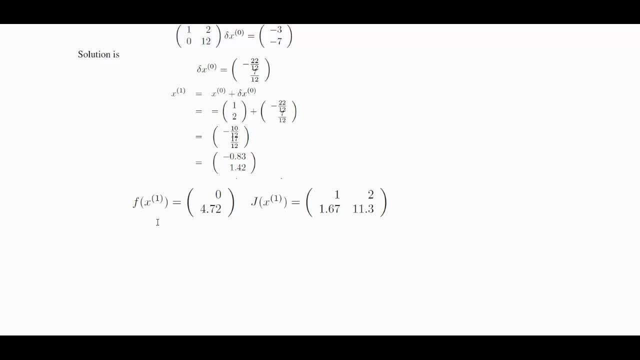 and of course next. so just here i'm showing you the, uh, the next iteration, so f of x1, some of the ingredients for it, so f of x1. and then we have, of course, that at x1, x2, uh, the, the, the first deterrent, now the updated one. so we are using these values minus 0.83 and 1.42. that gives us 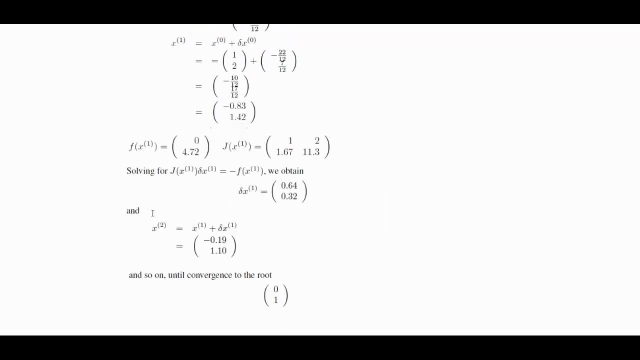 these two. so the jacobian at that then gives us this matrix. so basically, um delta x1 is 0.64.32, and of course we then calculate x2, which is equal to x1 delta x1, and of course here i'm talking about vectors. uh, we're still talking. 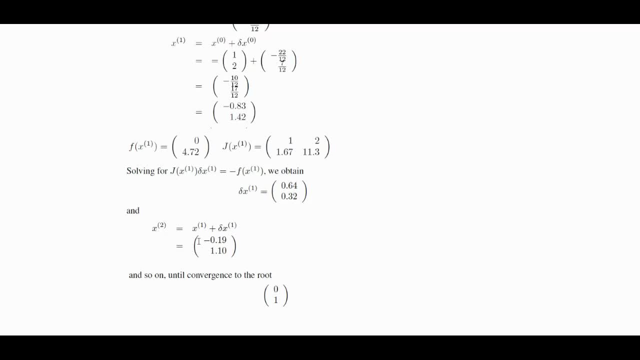 about vectors here. these are not single numbers, of course, um so anyway, that gives us this updated x2 vector and the second iteration, and we can continue this way until we reach the correct root, which is actually 0, 1.. so this hope, hopefully, this example demonstrates to you how the 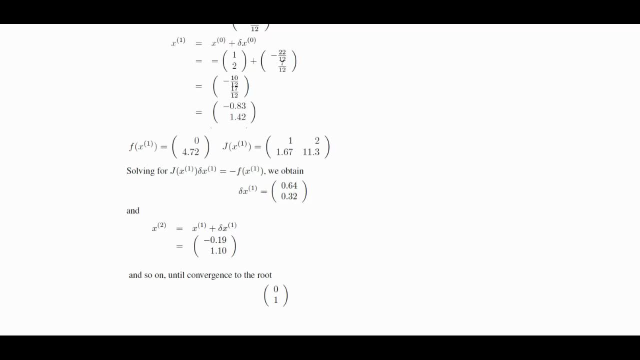 system of non-linear equations, how a system of non-linear algebraic equations can be solved using method adopted, adapted, sorry, for systems of non-linear equations. so final thoughts, uh, on this before we end. important thing to understand is that the jacobian matrix that we're calculating, 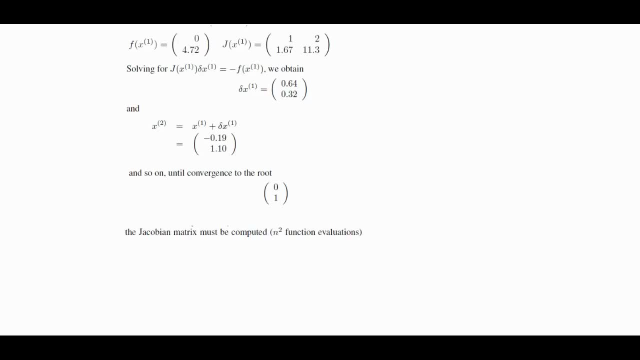 here requires approximately n squared function evaluations, and that's quite expensive. this makes this method quite expensive. one can actually show that in fact, this, the overall number of steps requires required is n cubed in fact. number of operations required is n cubed, which is quite expensive, in fact. now, 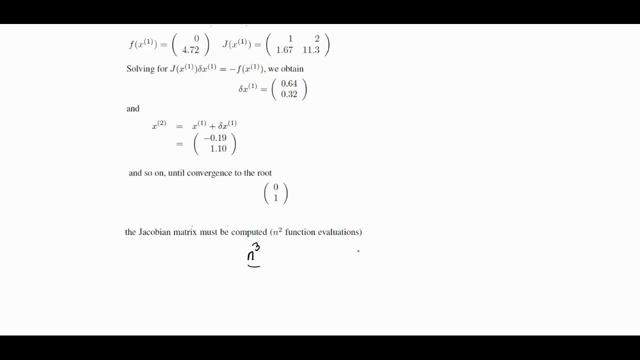 this sum of the expense can be cut down by using a uh, a version of the secant method which we used. uh, if you remember, earlier in this uh and and for the one-dimensional problems or single equations, uh. so the secant method was basically sidestepping. 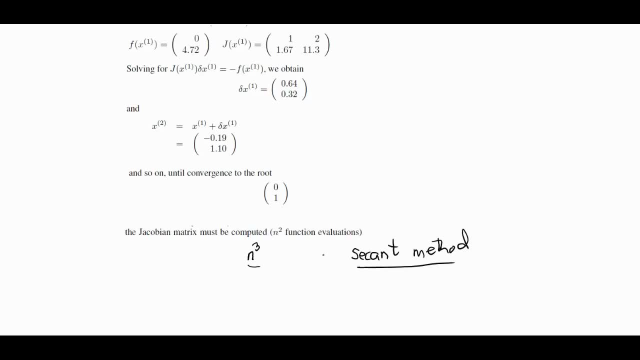 the calculation of the derivative. it's an approximation of the derivative that can be considered and it may be a little bit more complicated. but it's a little bit more complicated and it may lead to a slightly altered method which may be a little less expensive, uh, to calculate. 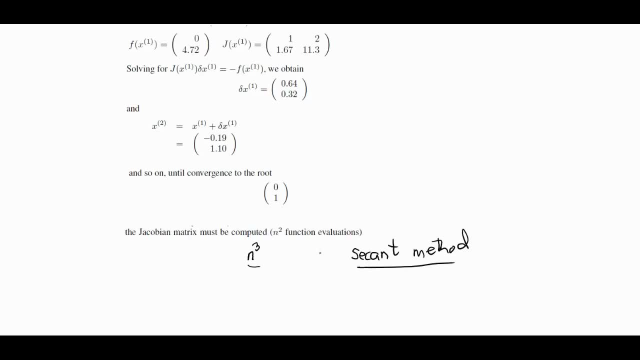 anyway. uh, with that, we will stop the this video and i hope that you understand how the newton's method, extended to um n dimensional or, um, sorry, a system of n equations and non-linear algebraic equations, can be employed.